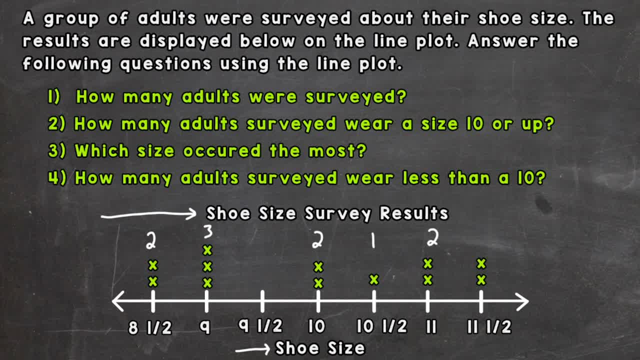 and for eleven and eleven and a half. I'm sorry, eleven and a half. we have two, so we need to count the total number there. add all those up to see how many people were surveyed. so two, five, seven, eight, ten, twelve. so how many adults were surveyed? twelve adults. 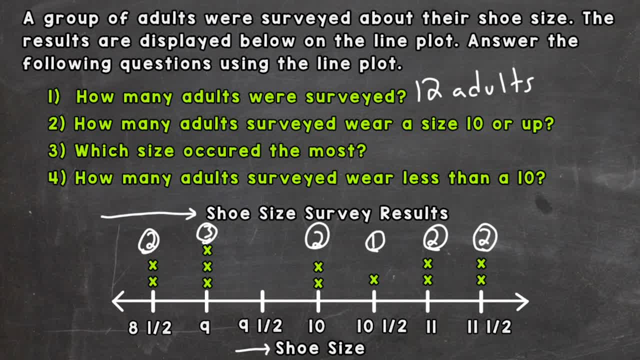 number two: how many adults surveyed wear a size 10 or up. so we need to include 10 and look at all the other sizes above 10. so it's going to be this portion of our line plot. so how many? well, two, three, five, seven, seven adults wear size. 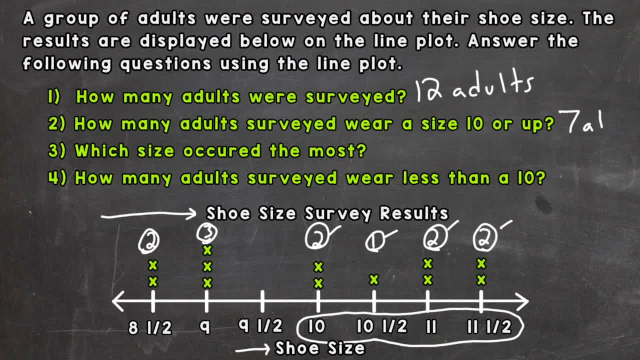 10 or up. oops, forgot my L there. number three, which size occurred the most. so let's take a look at what size has the most above it, which, again, those X's represent the adults that wear that size. so size nine has three people that wear it. that is the most occurring size. 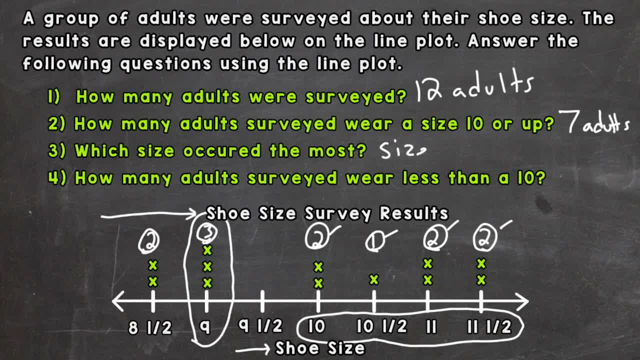 so it would be size nine. now number four: how many adults surveyed were less than size 10, less than a 10? so that does not include size 10 because we want less. so it would be this portion of our line plot and that includes two people for eight and a half and three people for size nine. 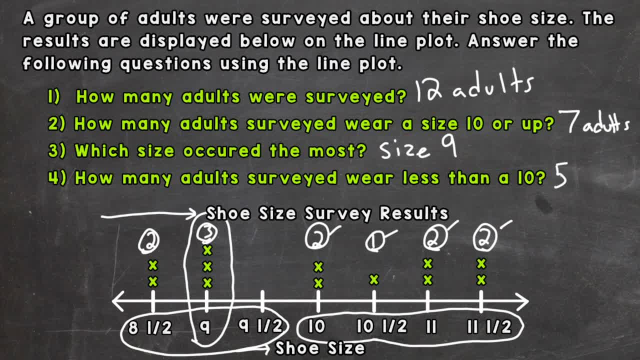 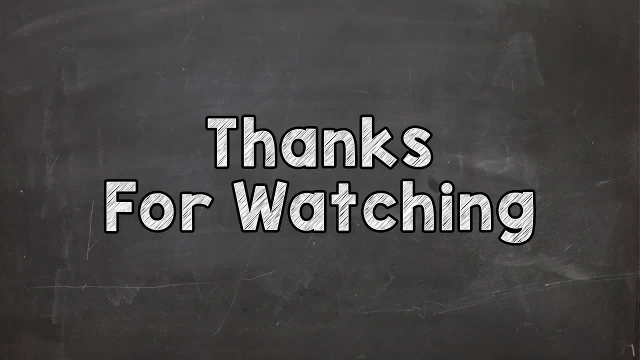 so that's a total of five adults wear less than a 10 as far as people surveyed for this line plot. hopefully that helps you guys. I hope you enjoyed this video and I'll see you next time. thanks so much for watching. until next time, peace.